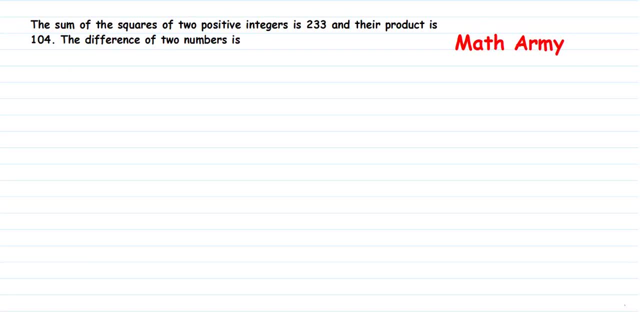 Hello guys, welcome to my channel, MathArmy. The sum of squares of two positive integers is 233 and their product is 104.. The difference of two numbers is okay, Guys. first of all, let us assume that the two numbers be x and y. So write a statement: Let the two numbers be x and y. 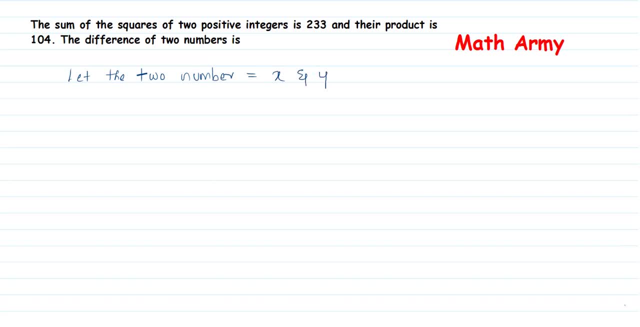 Now let us go back into the question. The sum of squares of. so what is the meaning of it? x square and y square add. So, given x square plus y square, is equal to 233.. And now- and they have given additional information- Their product is 143.. 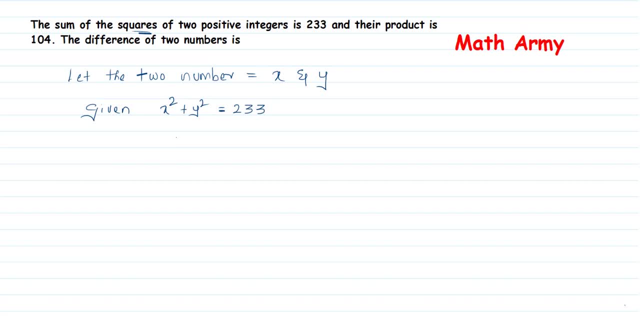 104.. So product means multiplication of the two numbers x and y here. So x multiplied with y is equal to 104.. Now what we are supposed to find? x minus y. Now take x minus y and square it. Yes, take x minus y and square it. 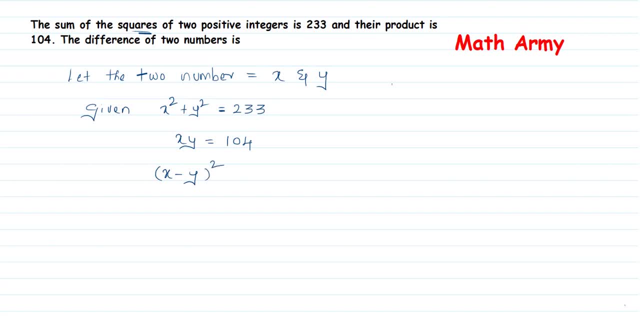 Yes, entire thing. And what is the formula of x minus y- whole square, Guys? if you don't know, so think of one of the identity: a minus b whole square. What is the formula? A square plus b? square minus 2ab right. 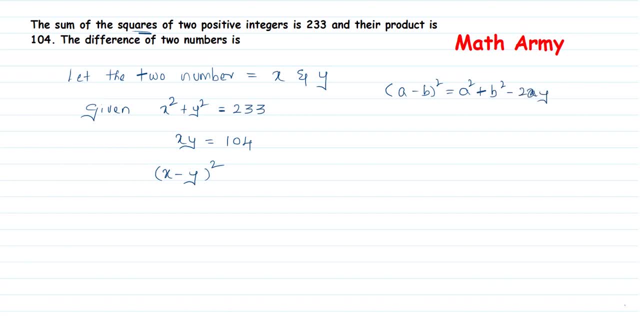 Not 2xy, guys, It is minus 2ab. Let me correct that. Okay, Now apply the same formula: A square plus b square Minus 2ab. So here it is x square plus y square, minus 2xy. Now what is the value of x square plus y square? It is 233.. It is given in the question itself, right, This one.